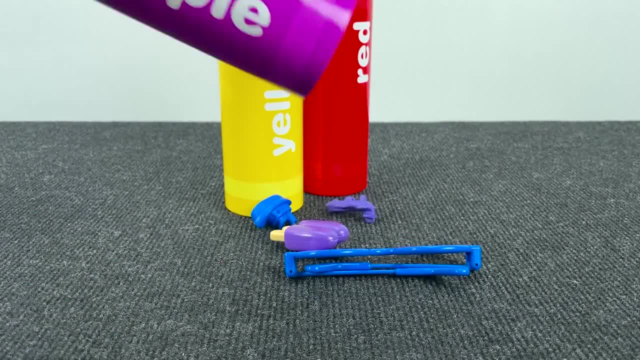 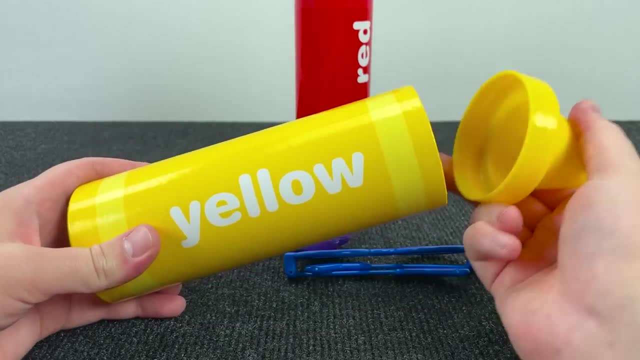 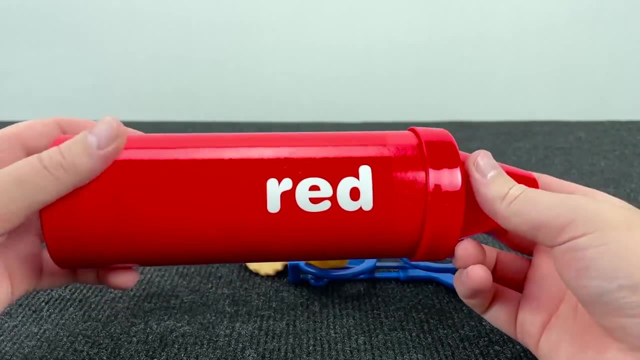 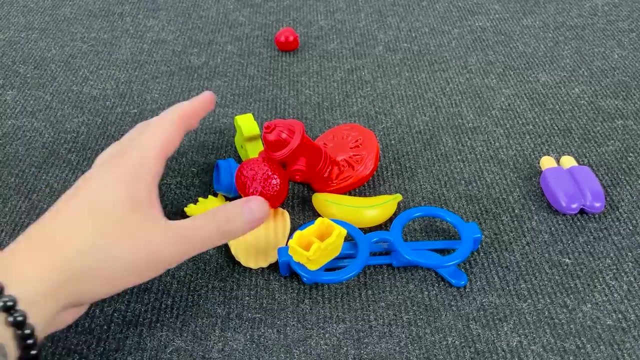 Let's see, Wow Again. no, Let's open yellow sourcing crayon now, Maybe here, Oh Again. And let's open last sourcing crayon. This sourcing crayon is red. Wow, You see, Number Nice, It's number four. 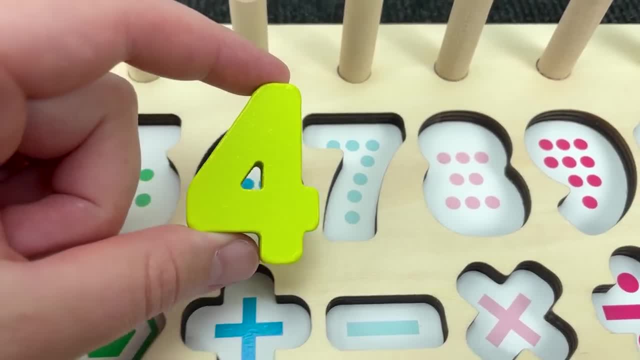 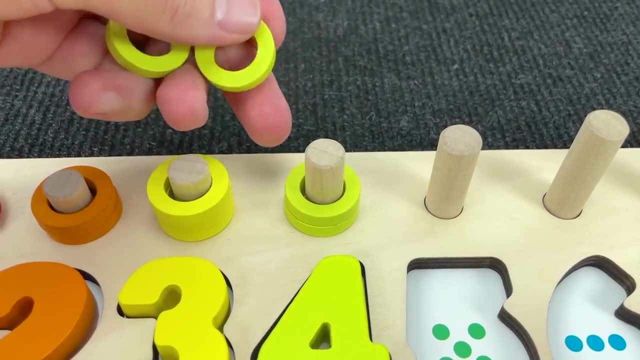 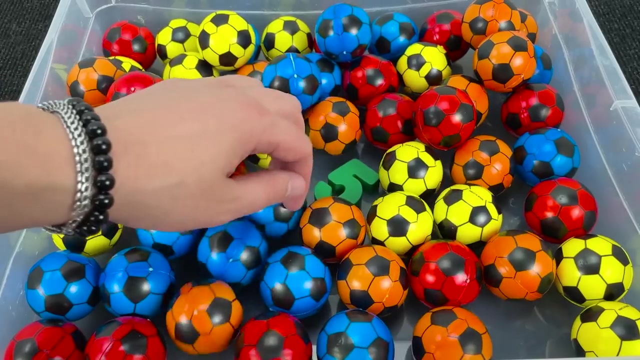 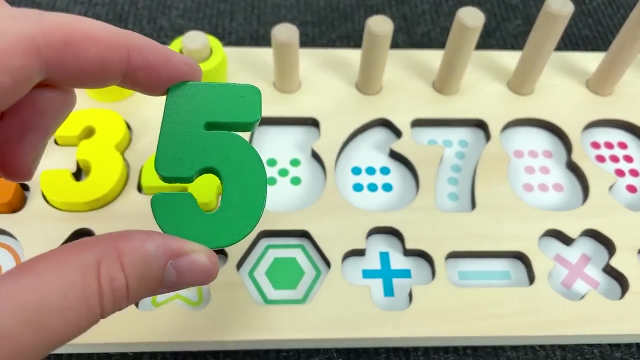 Number four. Where should I put No Right? And here four dots: One, two, three and four circles. Wow, How many soccer balls. Where next number Right? It's number five, Green number five, Where this number You're right. 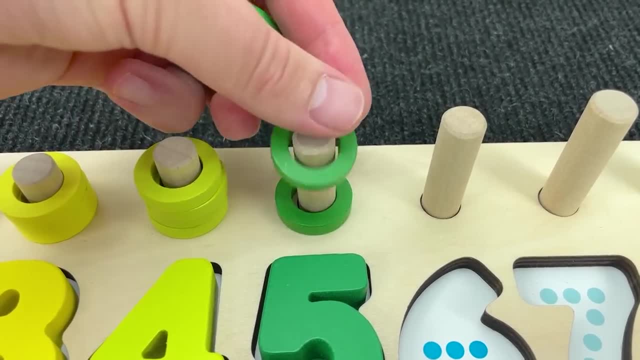 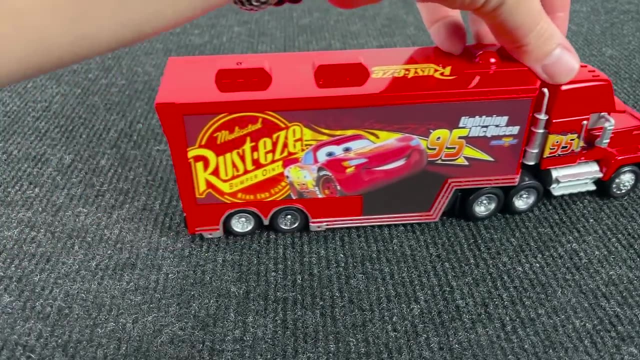 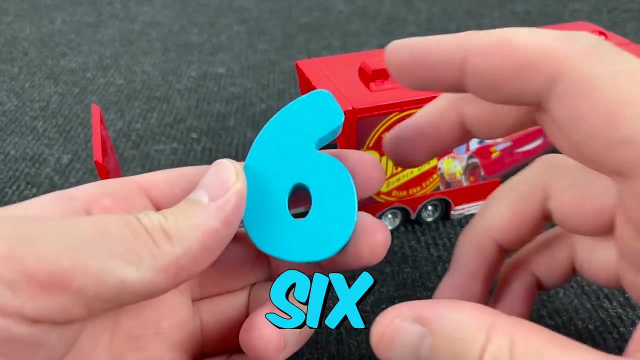 Here five dots: One, two, three, four and five circles. Wow, It's mug. Let's see what's inside. Oh, It's number six, Blue number six. Can you help me find this number? No, No. 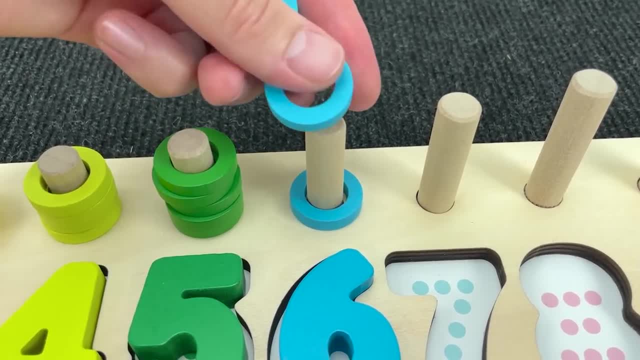 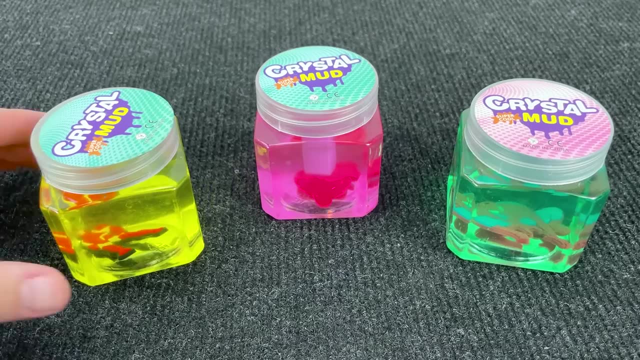 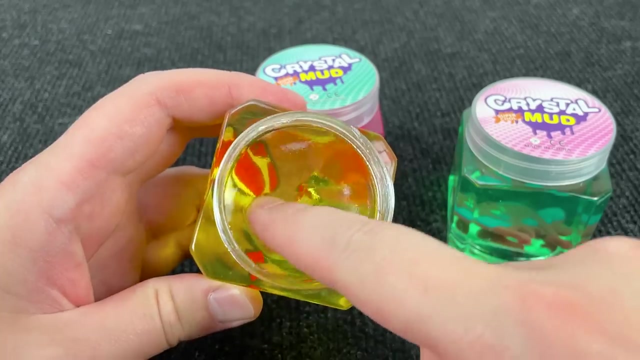 Right, And here six dots: One, two, three, four, five circles. One, two, three, four, five and six circles. Wow, It's slimes. Let's see what's inside: yellow slime And here iron man, But no number. 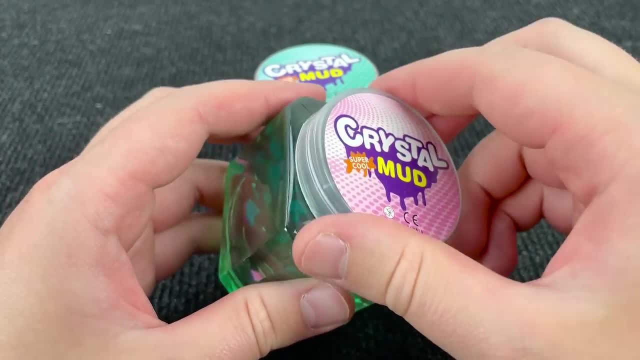 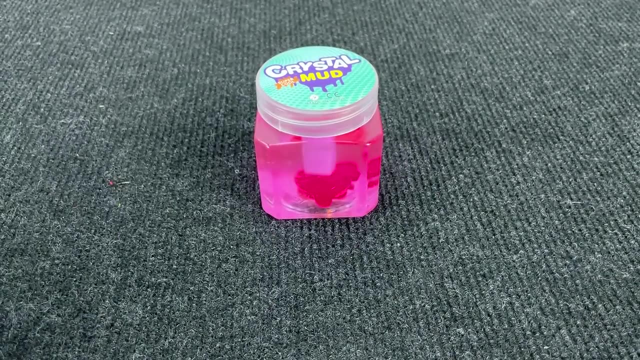 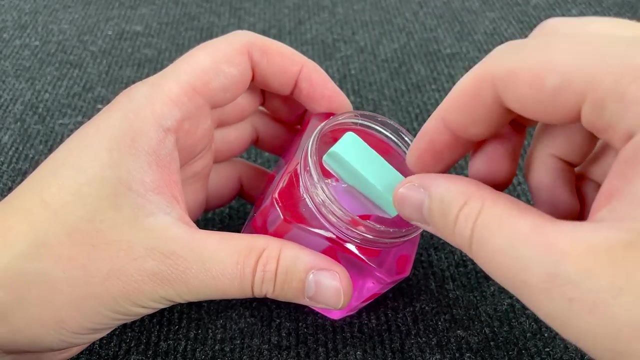 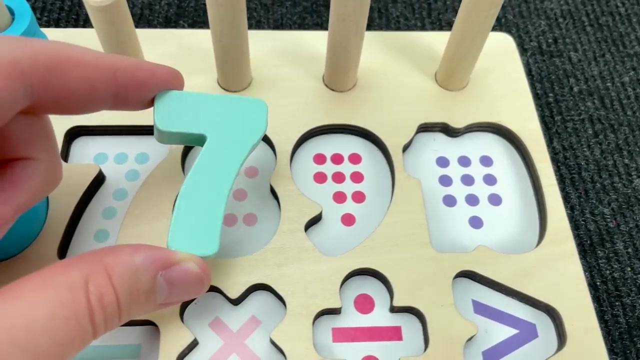 Let's see what's inside. turquoise slime, Maybe here, number Oh no, Here spider man. Now let's open pink slime, Maybe here, Oh nice, And it's number seven. Number seven, No, No Right, And here seven dots. 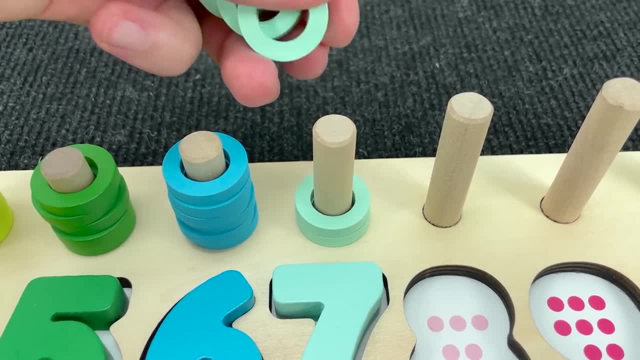 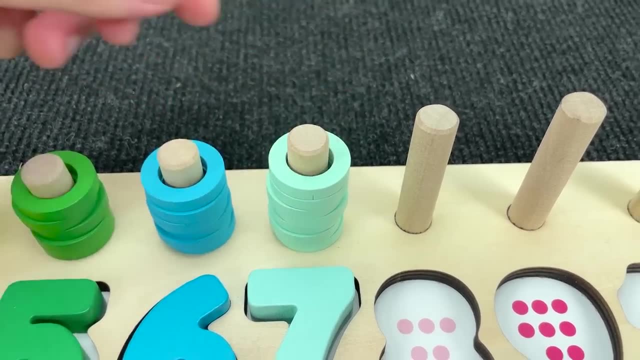 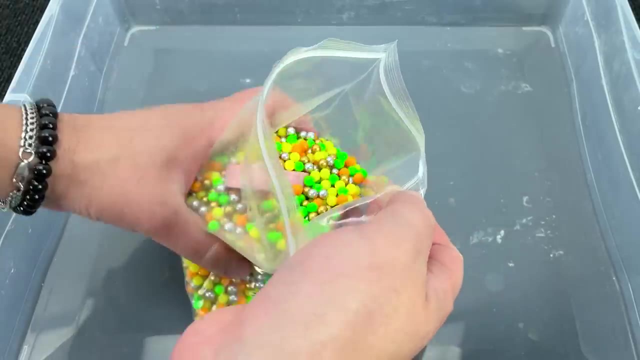 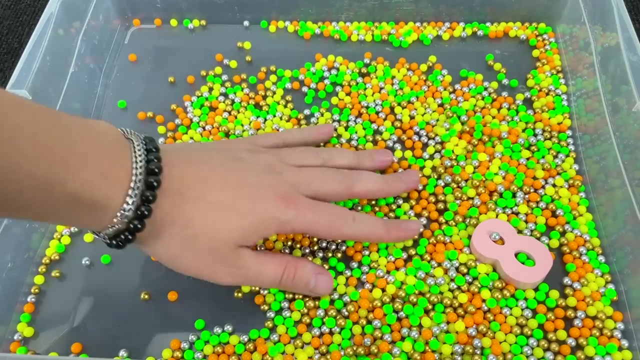 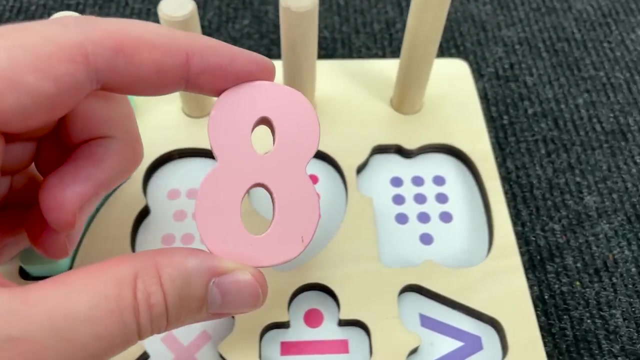 One, two, three, four, five, six and seven circles. How many little colored balls. Let's find next number Open. Wow, You see next number Right, It's number eight. Number eight, Where should I put? 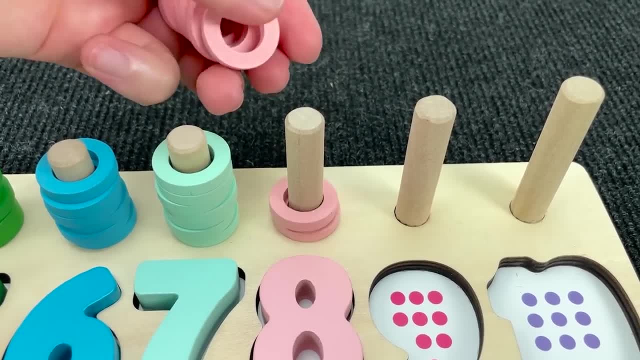 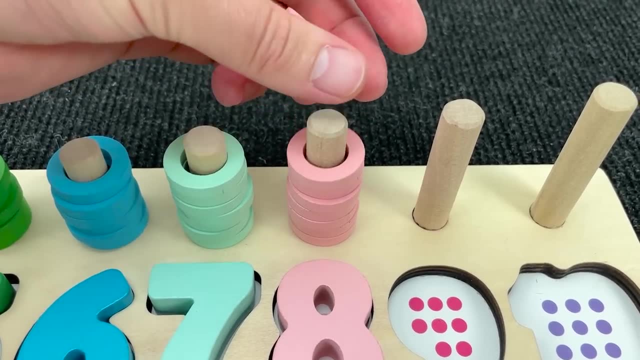 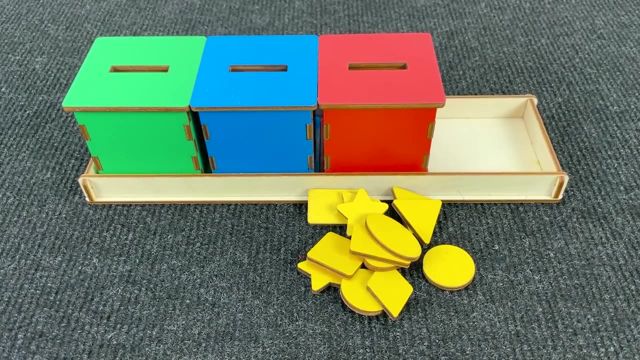 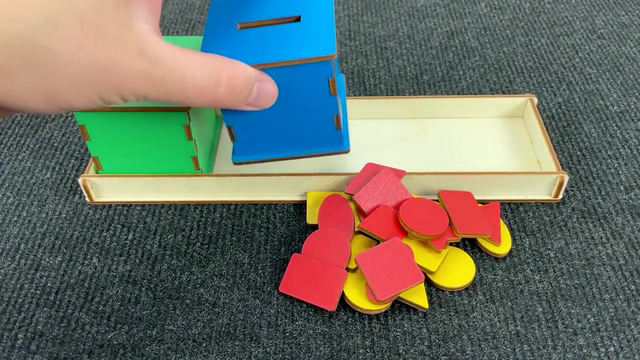 Oh good, Yeah, One, two, three, four, five, six, seven and eight circles. Wow, Here colorful boxes. Let's open yellow box And here no number. Maybe inside red box Again. no, Let's see what's inside blue box. 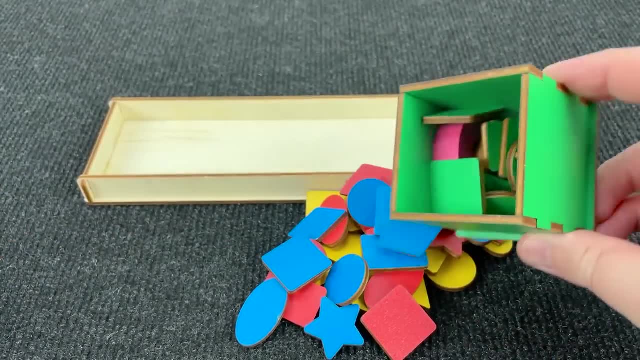 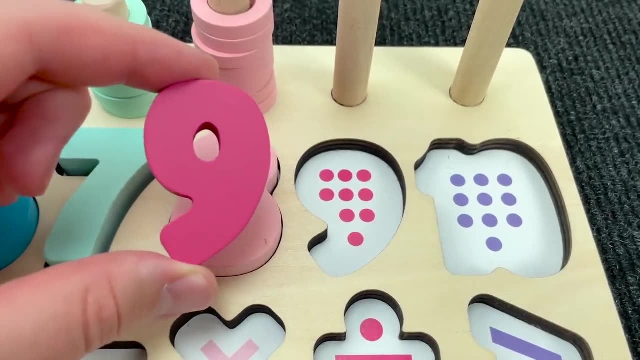 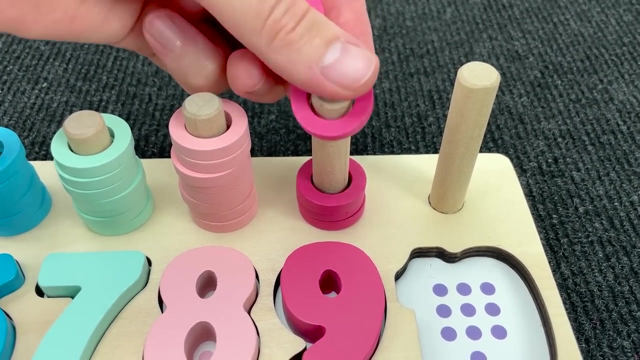 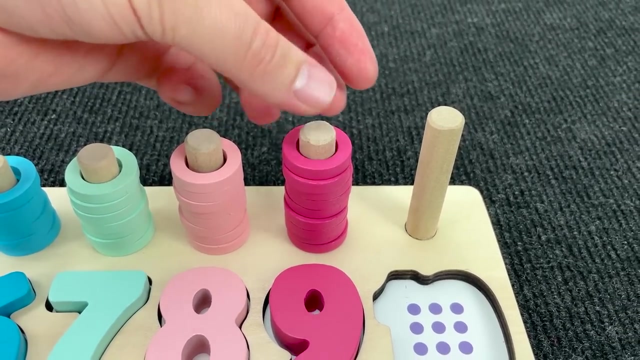 Oh, again And last, this box is green. Oh nice, It's number nine, Number nine. Let's put this number here: One, Two, Two, three, four, five, six, seven, eight and nine circles. Oh, it's glossary basket. 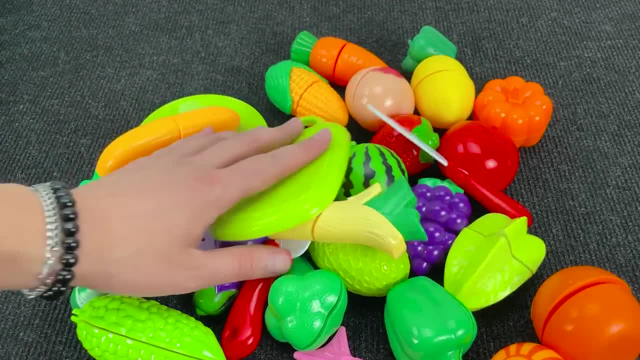 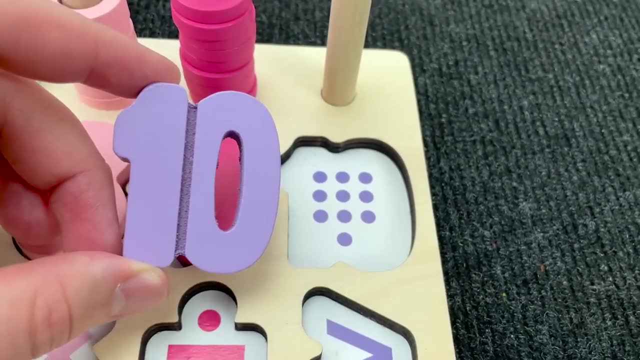 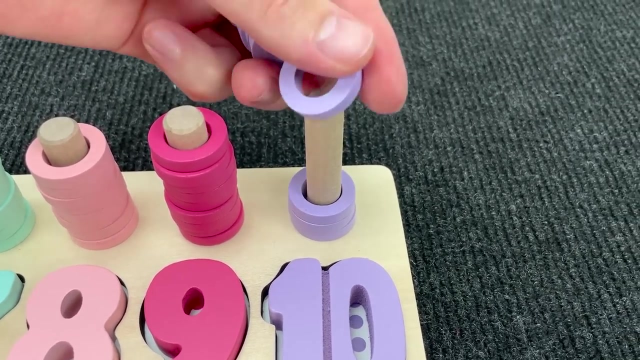 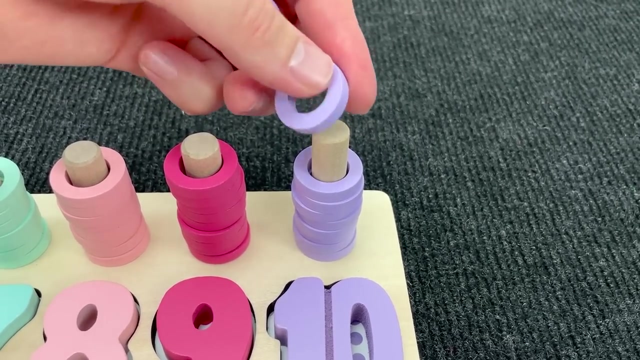 Let's find next number. You see next number? Oh nice, it's number ten, Number ten. Let's put number ten here: One, two, three, four, five, six, seven, eight, nine and ten circles. 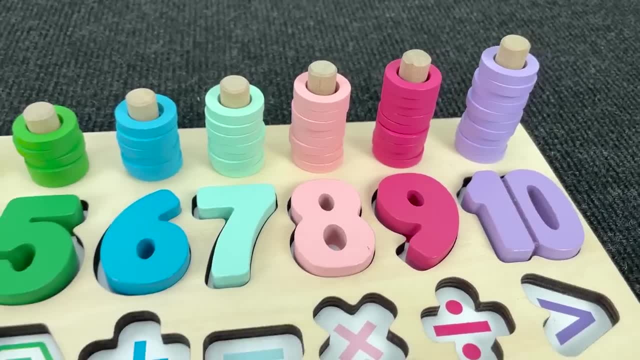 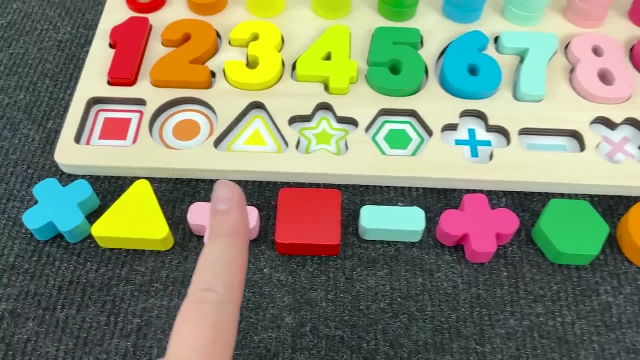 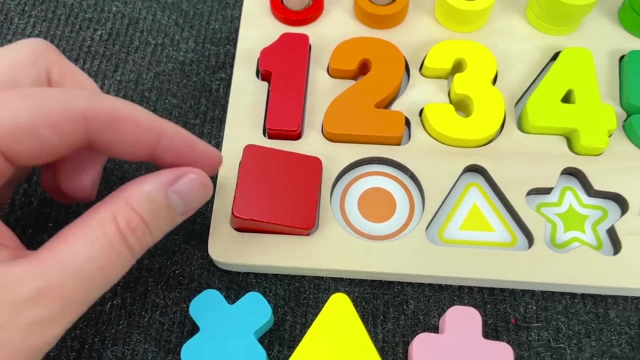 Wow, we did it. We found all numbers. And now let's placing these shapes in the right places. Let's start with the square. Can you help me find square? Right, it's red square. Let's put square here. Now let's find circle. 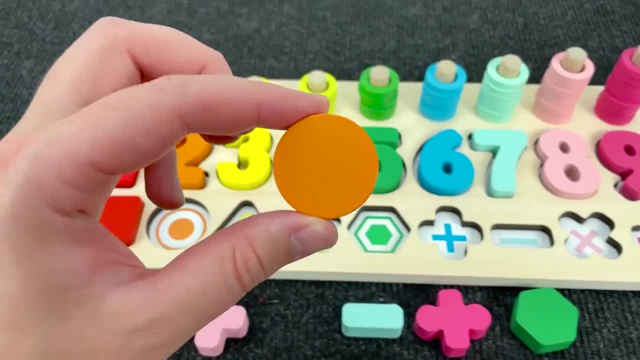 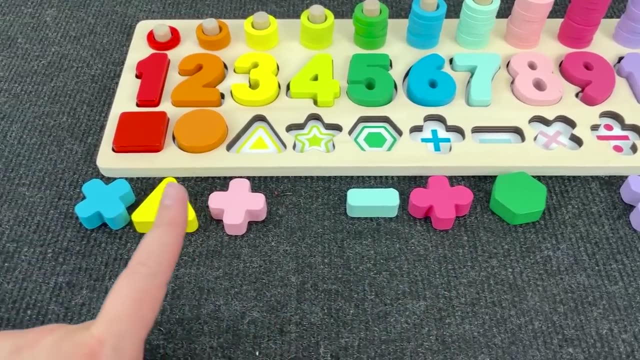 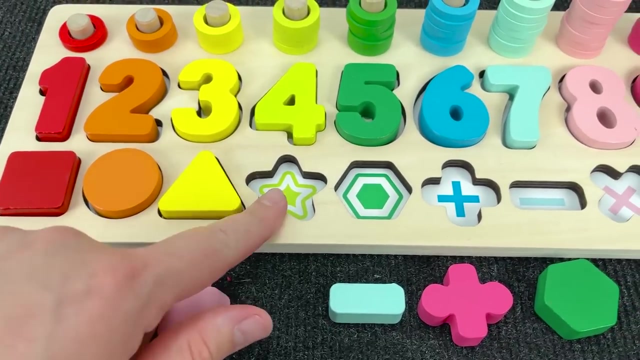 We need find circle. Right, it's orange circle. Let's put circle under number two. And now let's find triangle. You see triangle- Right, it's yellow triangle. And now let's put triangle under number three. And now we need find star. 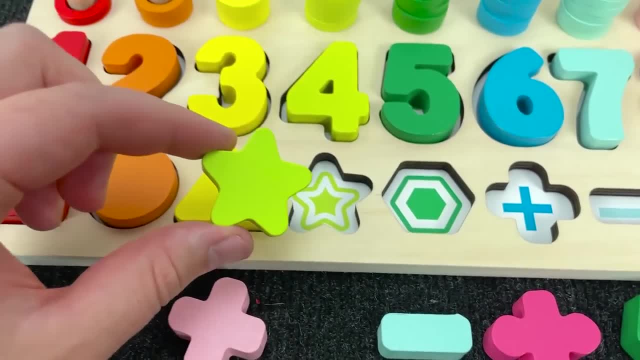 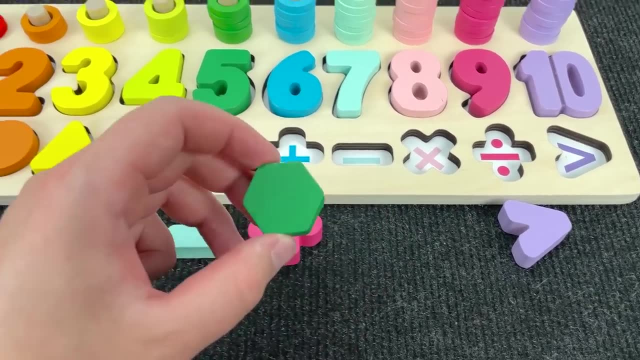 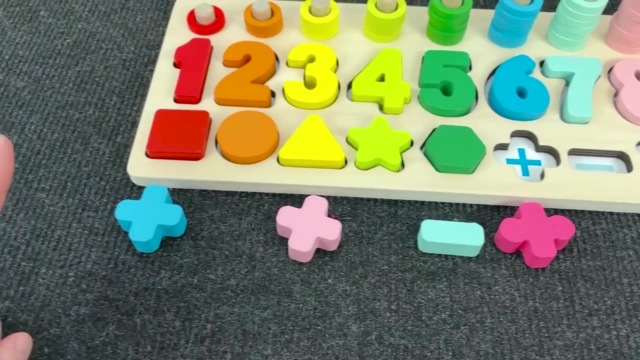 Nice, It's a star. Let's put star here. And now can you help me find hexagon? Oh, very good, Let's put hexagon here. Now we need find plus sign. Where plus sign? You're right, It's blue plus sign. 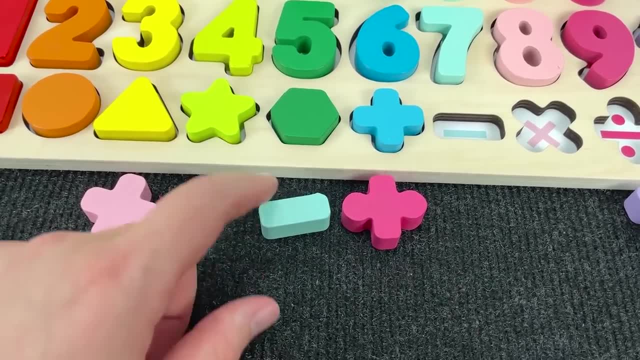 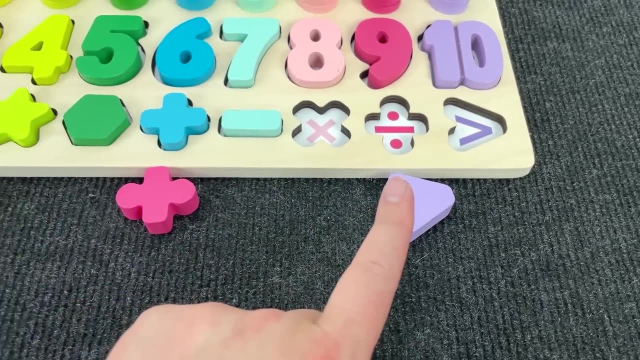 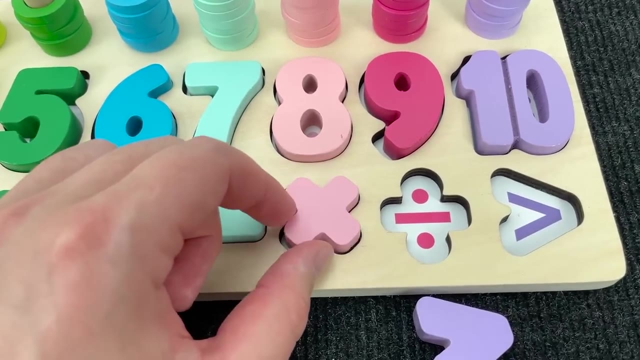 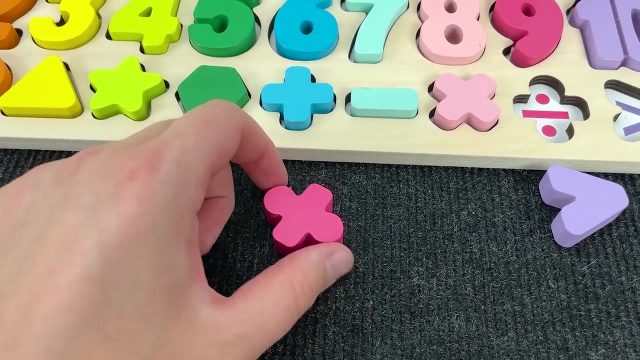 And now let's see where minus sign- Right, it's minus sign. And now we need multiplication sign- Right, it's multiplication sign. And it's division sign. No, Right, it's division sign. Let's put it here. 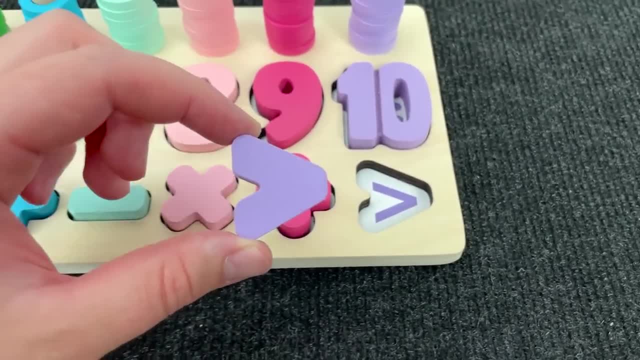 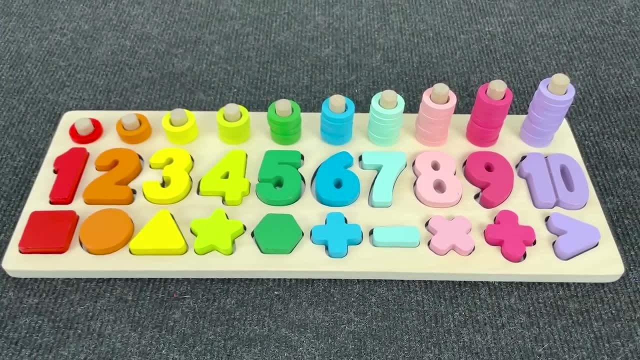 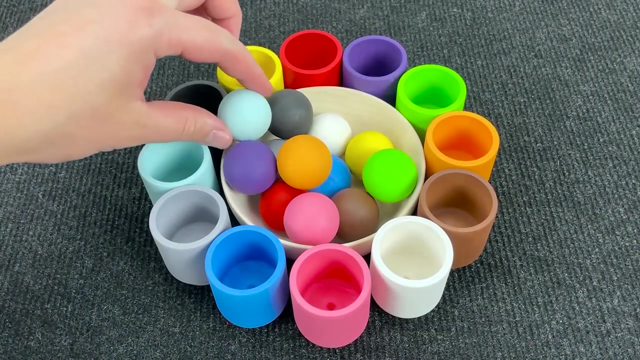 And last, it's more sign. Let's put more sign here. Oh nice, Congratulations, Congratulations. And now let's go to the next puzzle. And now we have colorful cups and colorful balls. Wow, Let's take first ball. 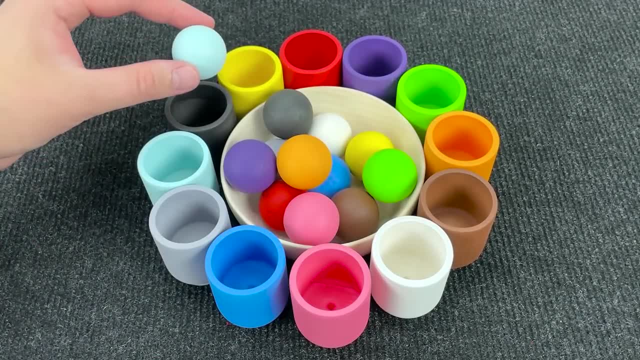 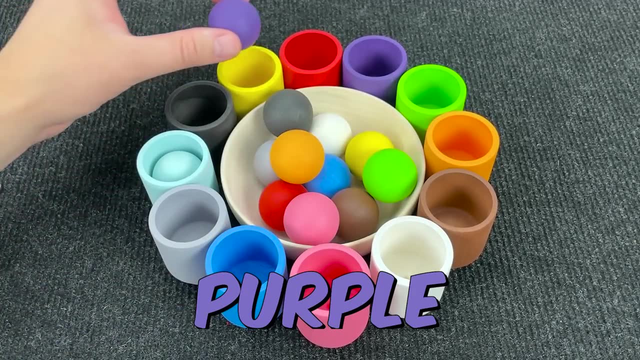 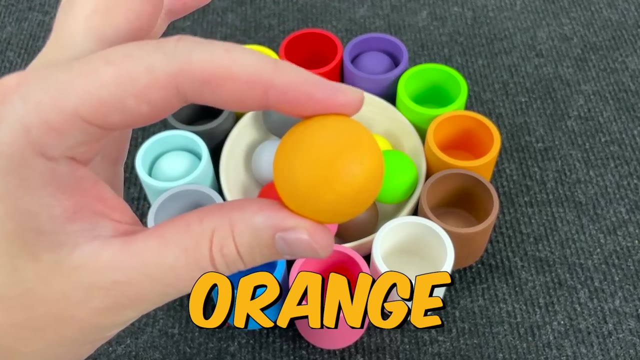 This ball is light blue. Where shall they put? Right in the light blue cup. Next ball is purple. Can you help me find right cup. Right in the purple cup. What next? Oh, this ball is orange. Where shall they put? 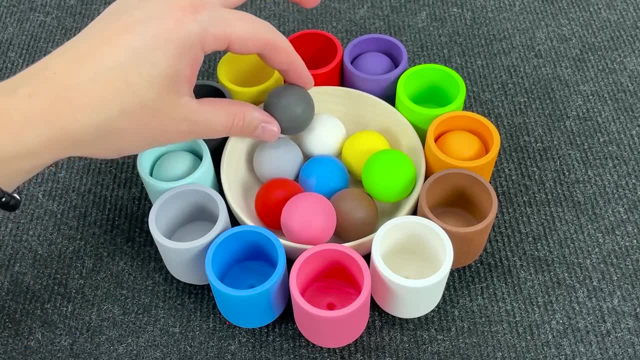 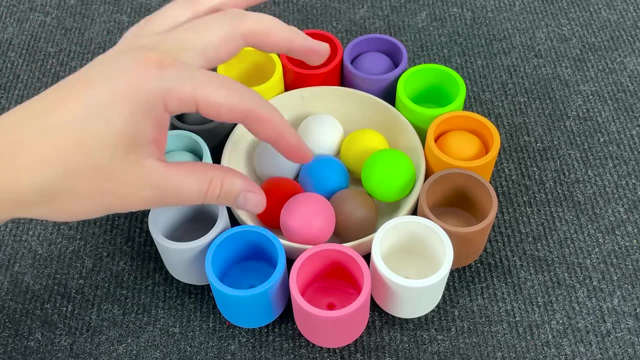 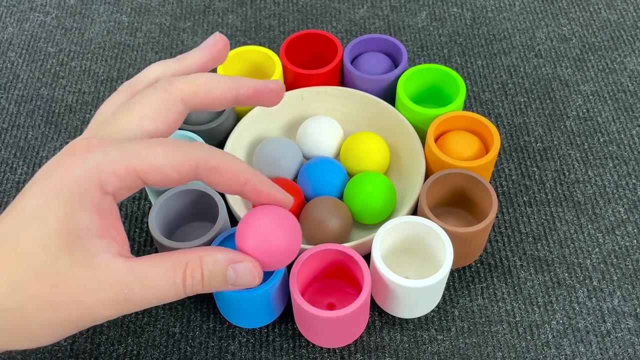 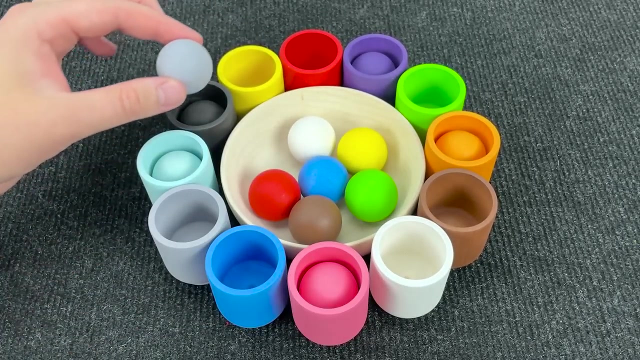 Right in the orange cup. Right in the orange cup. Next ball is black. Where black cup. You see, Right Next ball is pink. Can you help me find pink cup? No, Right Next ball is gray, Where gray cup. 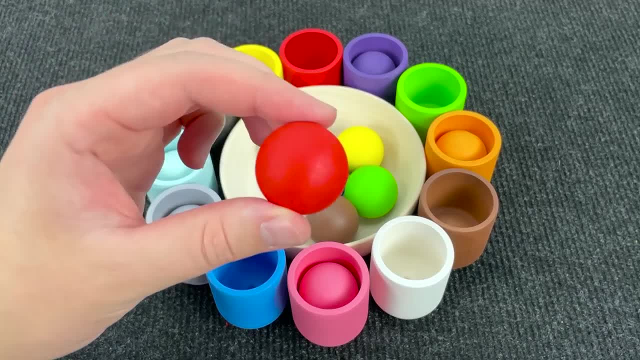 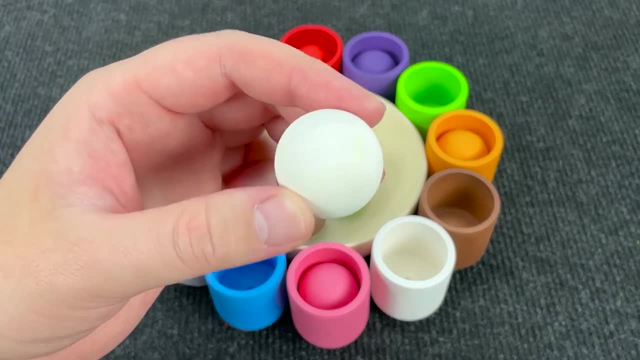 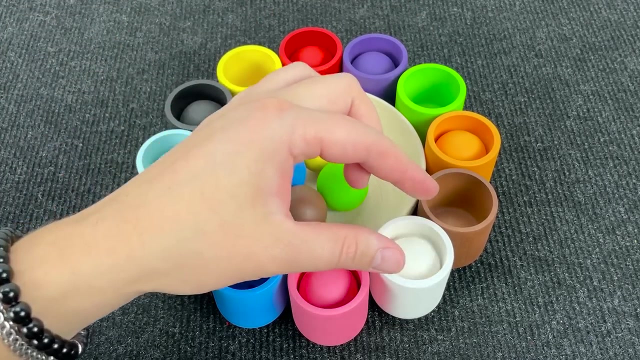 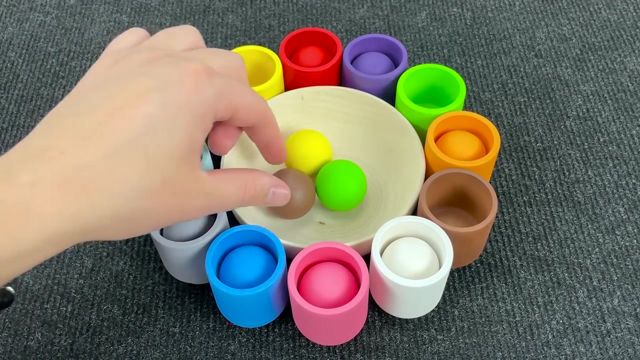 Hmm, Right, Next ball is red. We need to find red cup, Nice. And now we have white ball And we need to find white cup. Where white cup? Right? And next ball is blue, Where shall they put? You're right. 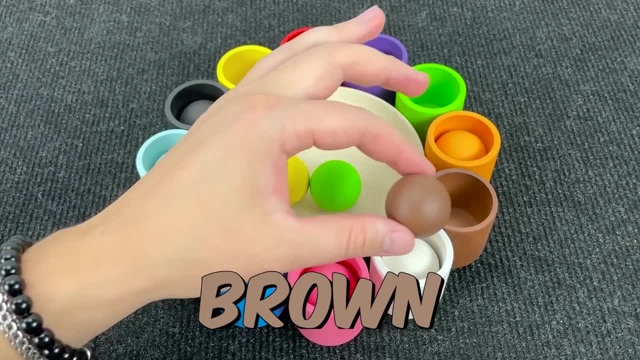 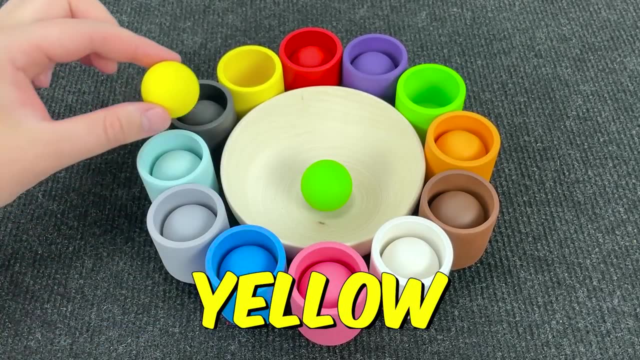 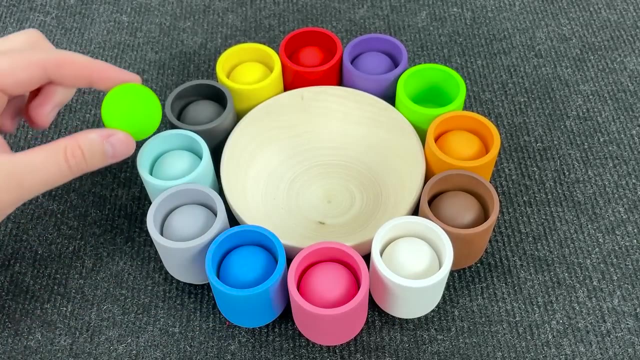 And now we have brown ball- Where brown cup? You're right. And this ball is blue. And this ball is yellow. Where yellow cup? Nice. And last ball is green. Where shall they put? You're right in green cup. 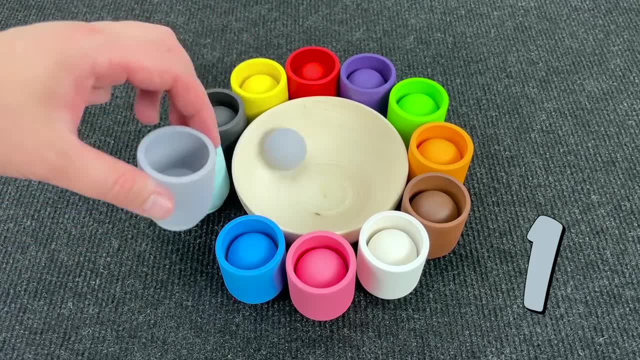 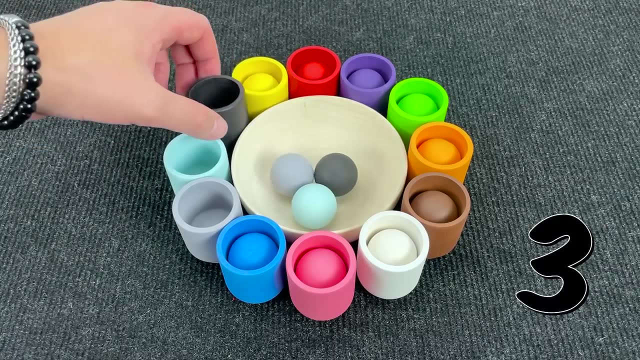 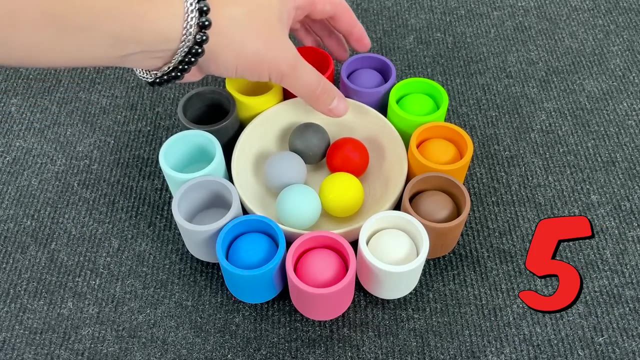 Now let's count. One It's gray, Two It's light blue, Three is black, Four It's yellow, Five It's red, Six It's purple, Seven It's green, Eight It's orange. 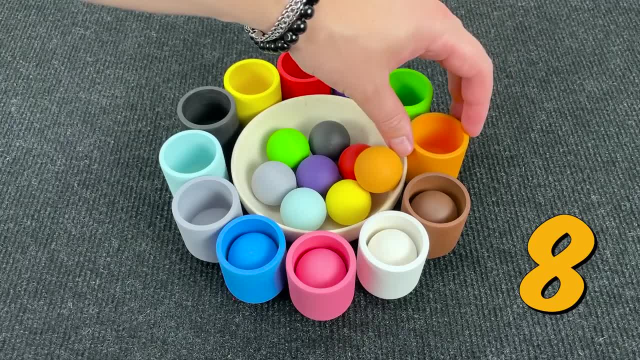 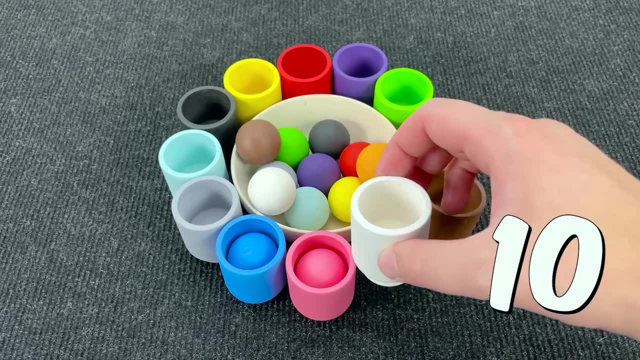 Nine It's brown, Ten It's white, Eleven It's pink And twelve It's blue. Nice, Now let's make a little mess. Wow, Very good. One, Two It's green, Three It's yellow.